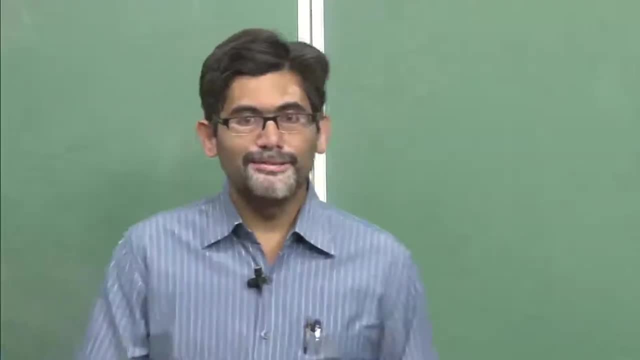 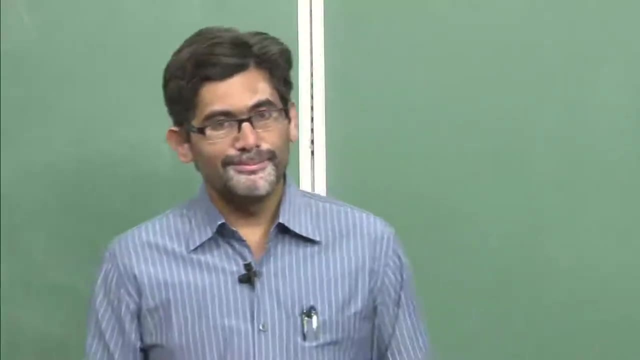 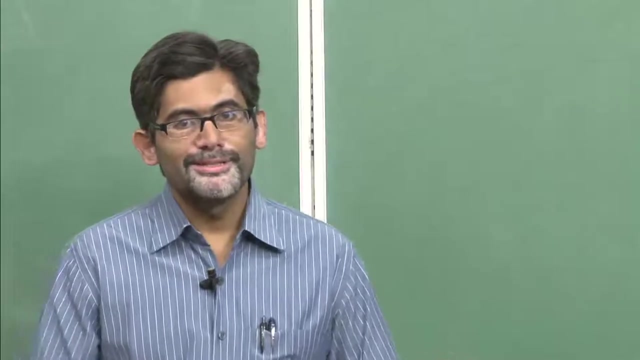 I am going to talk about in this course, but basically I will be giving you some kind of idea about these three important theorems. So I will be talking about completeness theorem, which is due to a famous logician, Kurt Gödel, And then I will be talking about one of the important theorems, which is known as compactness. 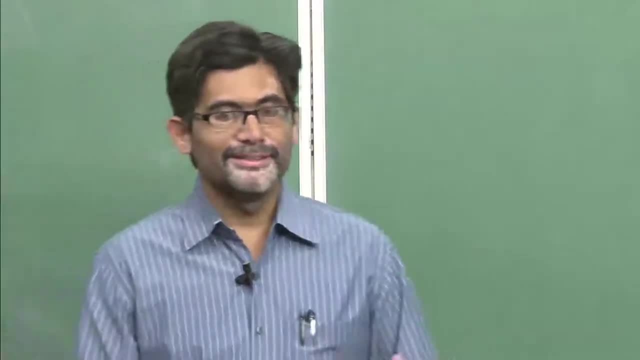 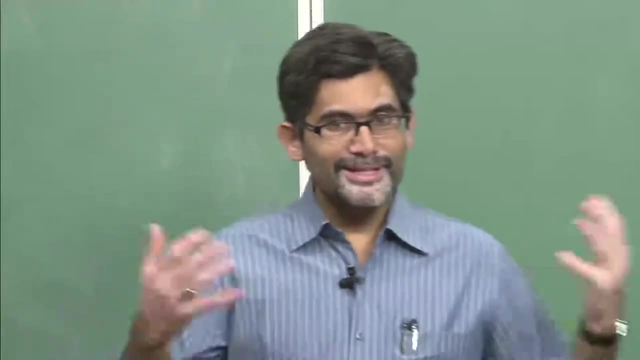 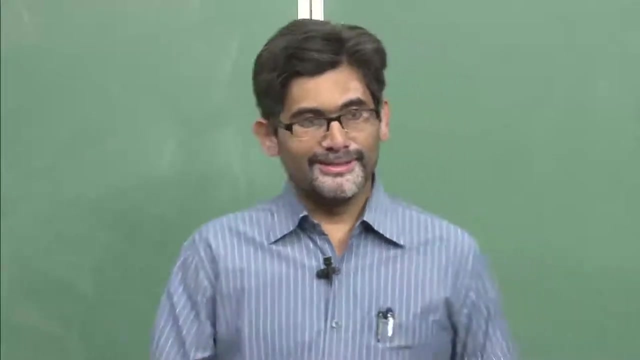 theorem. and third, one which is discussed widely in the literature of logic, and no course of logic would be complete without this celebrated result. so that is the Gödel's incompleteness theorem. So Gödel has been credited for both the completeness theorem as well as the negative. 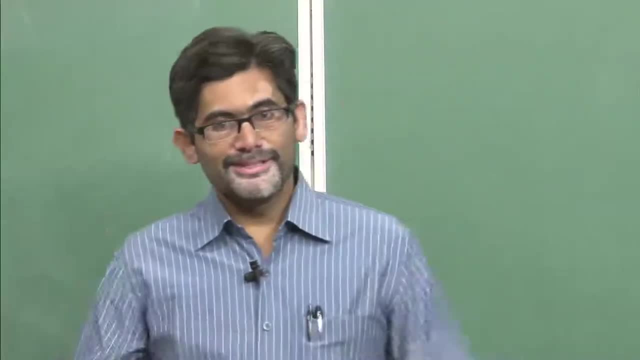 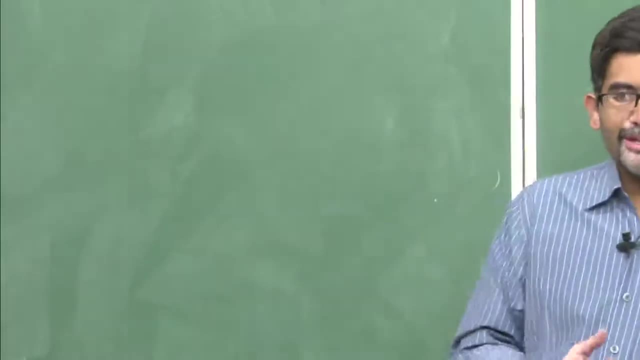 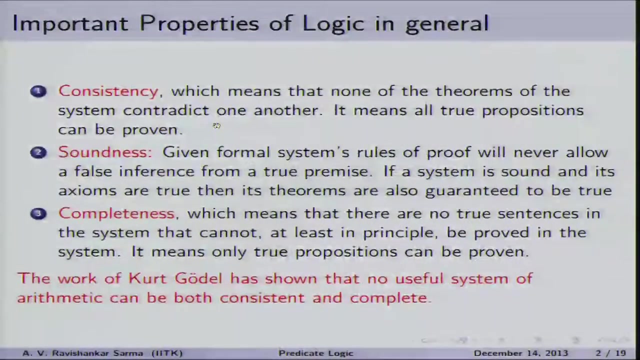 result. that is, incompleteness theorem. Incompleteness theorem is used widely used, misused and even sometimes even abused also. So we will be talking about some of the basic ideas of these particular kinds of theorems in this lecture. To start with, before going any further, we need to know something about. 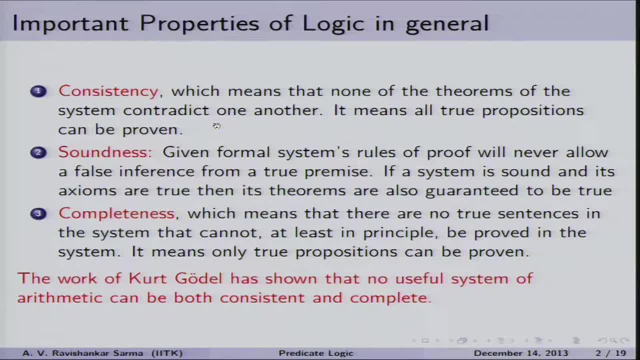 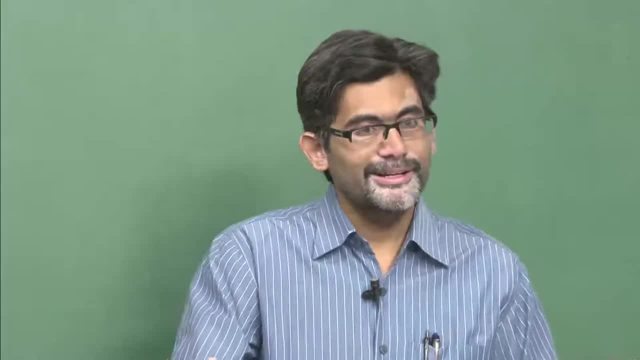 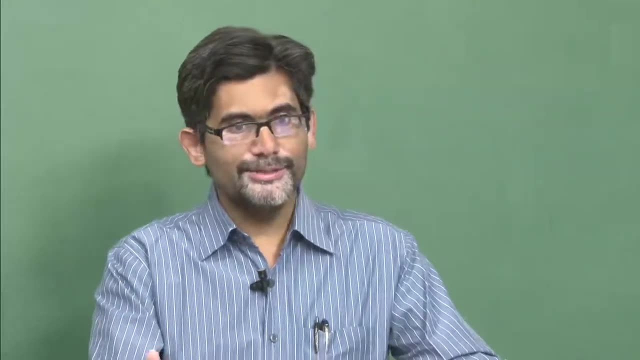 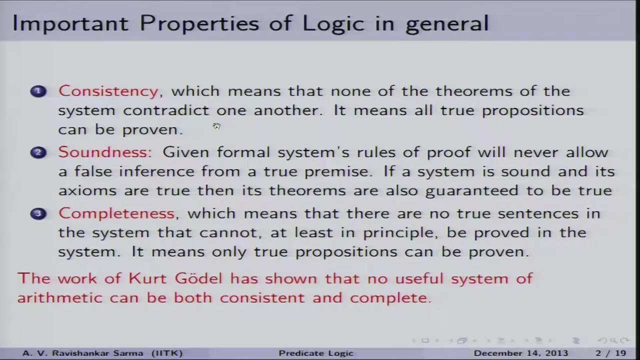 these three important logical properties. So any logical formal system, any logicians dream is to have these three particular kinds of properties. So in this course is all about the first order logic, which includes predicate and propositional logic. The one of the important characteristics of first order logic is that first order logics are considered to be consistent. 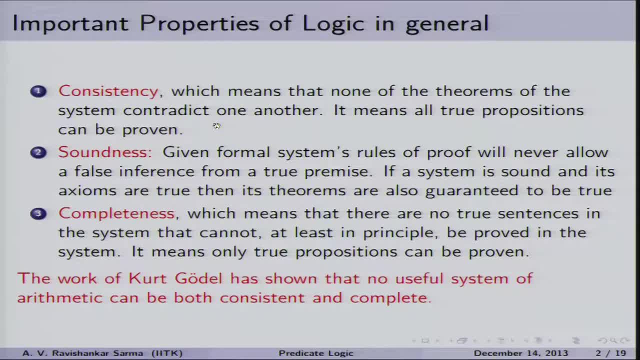 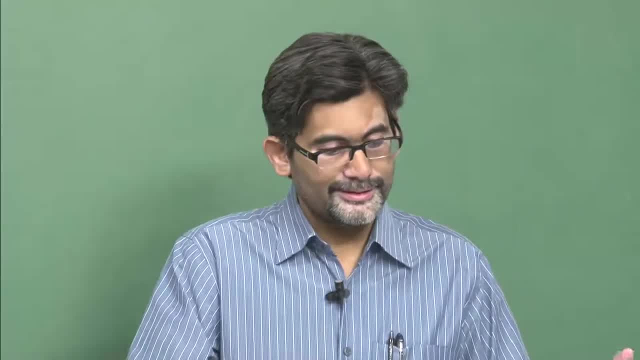 they are considered to be sound and they are also considered to be complete. When you come to second order logics, et cetera and all, it is very difficult to establish the completeness properties. So now, what are these important logical properties? we will just go through some kind of detail. 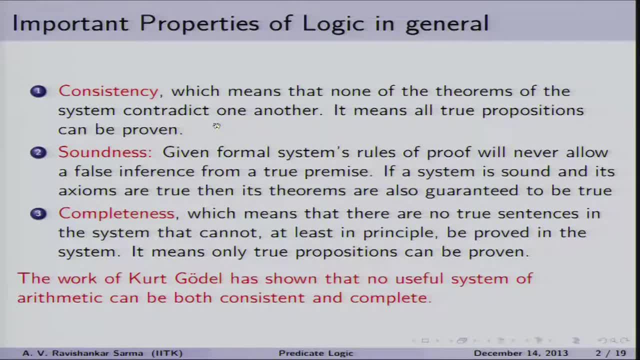 about these important logical properties all the time. we are using these three properties when we are, while we are discussing about semantic, tableau's method or natural reduction method, etc. So, consistency: if the first property is consistency, consistency means that none of the theorems of your formal system contradict one another. so that means you are not in a 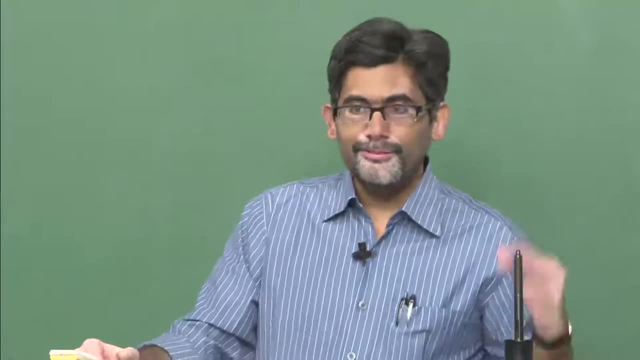 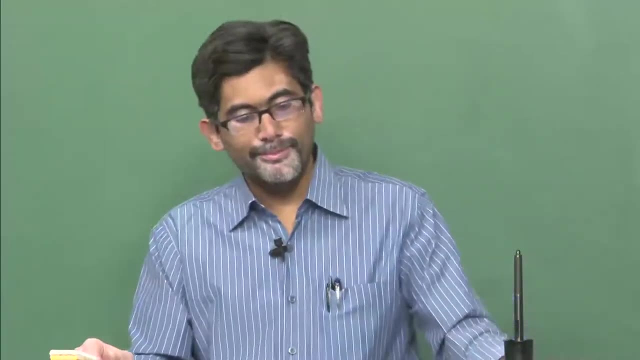 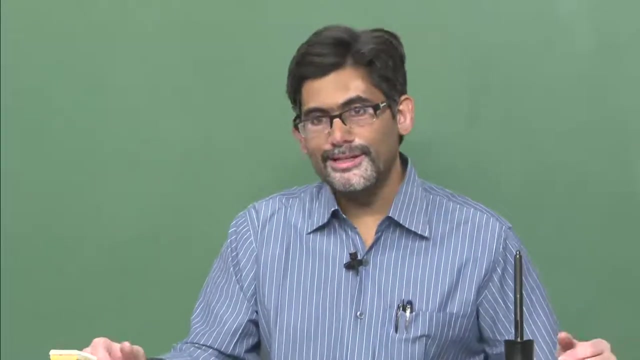 position to derive both P and not P. you know, if you derive both P and not P, then your system is considered to be consistent. so that means all true propositions can be proven. for example, if some something is a true proposition or true formula, that is tautology, all tautologies. 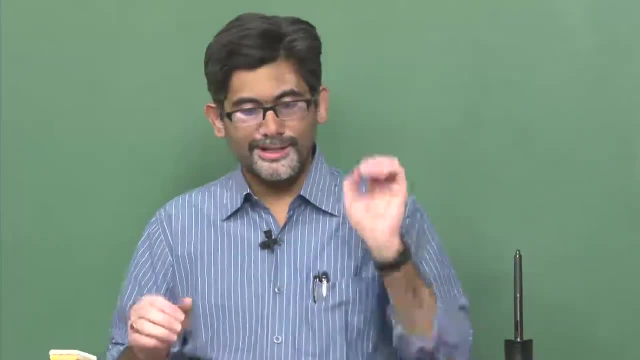 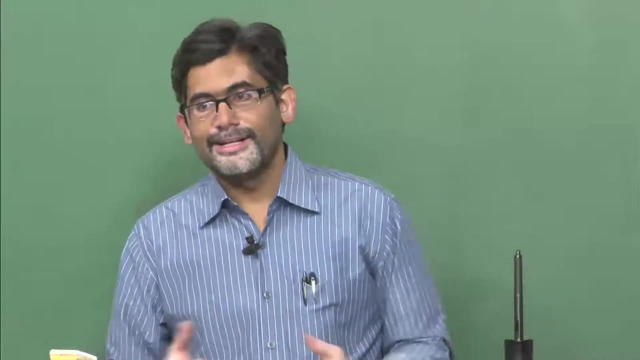 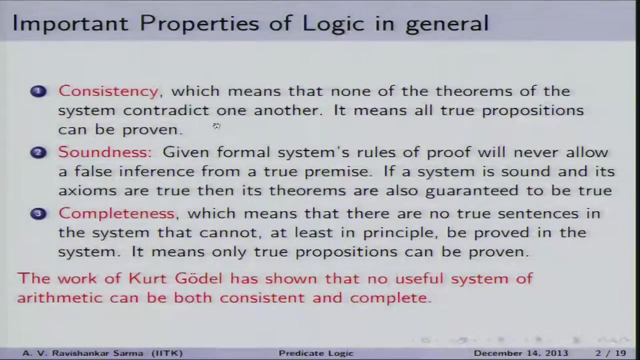 are obviously valid formulas and all valid formulas have to. we have to find a proof for all the valid formulas. in that context we use natural reduction and some other semantic tableau's method, etc. We already done those things. second important property is soundness. the soundness property tells us that a given formal systems, rules of proof will never allow. 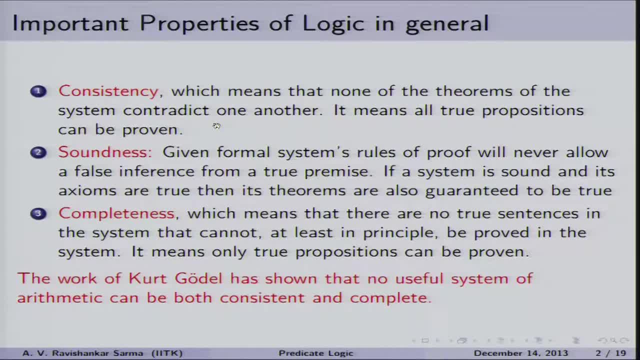 us false kind of inference from the true premises. if you start with the true premises, you always end up with a true conclusion, or there is no way you can generate a contradiction when you start with tautologies. So that is the reason why we have cleverly chosen axioms into consideration and then 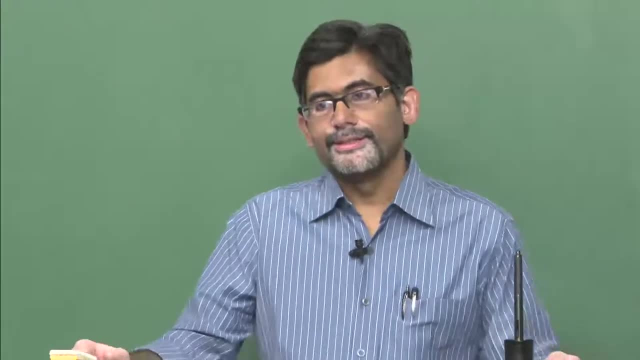 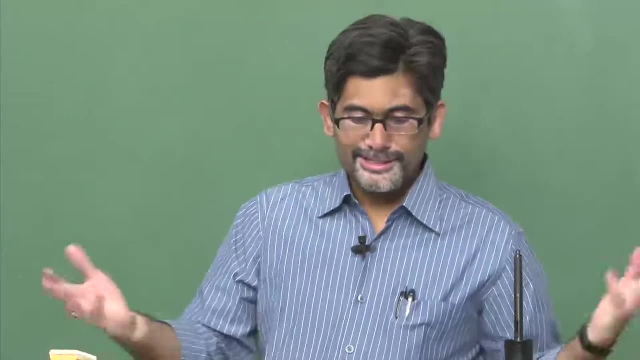 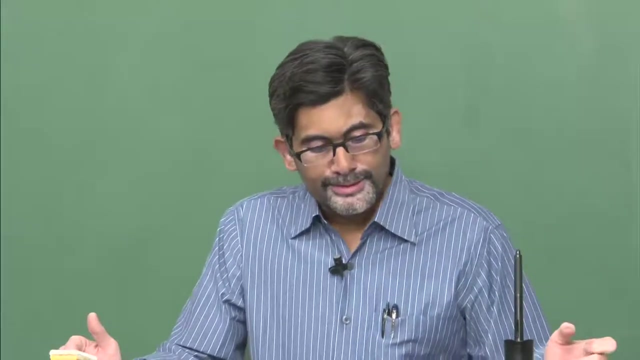 transform by means of substitution, rules, etc. and all modus ponens, etc. and then you, it will become theorem. all the theorems are also considered to be true. each step of your proof is considered to be true. the final step of your proof is also considered to be true. 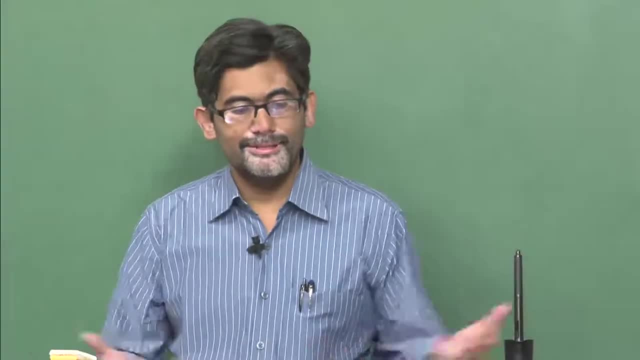 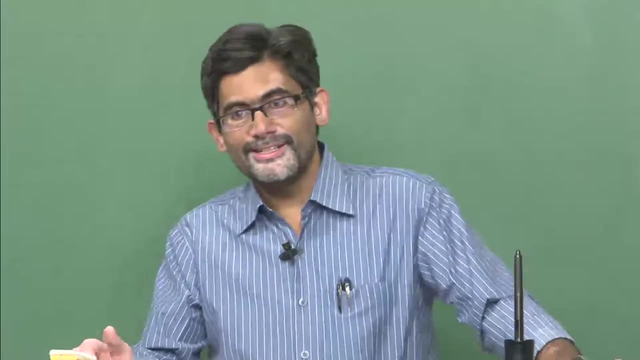 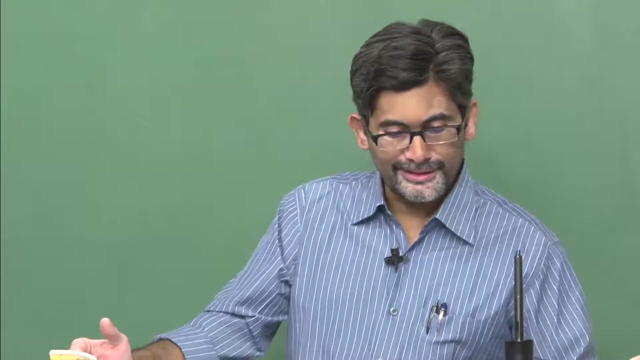 soundness ensures that you start with the axioms, which are obviously true tautologies, you will never end up with contradictions. so if you start with tautologies and end up with contradictions, something wrong with your formal System is something wrong with the proof, or there is something which is mistaken and all. 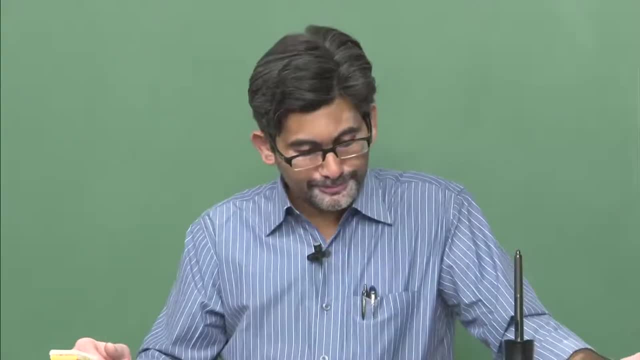 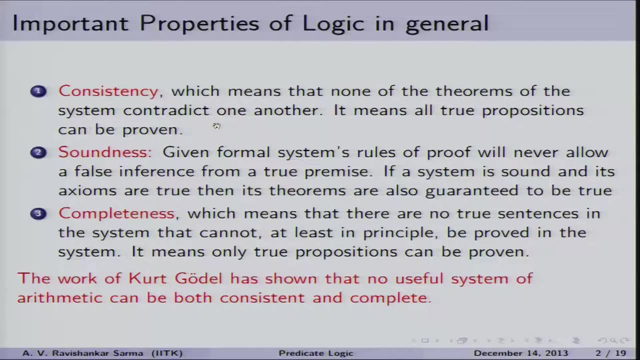 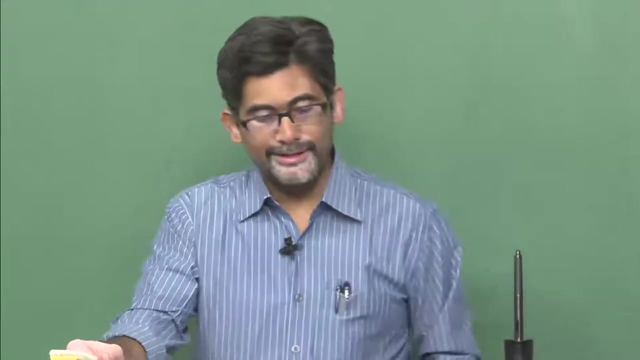 in the proof mistakenly considered. in the proof, the third important property is completeness, which means that there are no true sentences in the system that cannot, or at least in principle, be proved in the system. suppose, if you say there is something is a true proposition, it has to find a proof. that means we are also ensuring that only true propositions will. 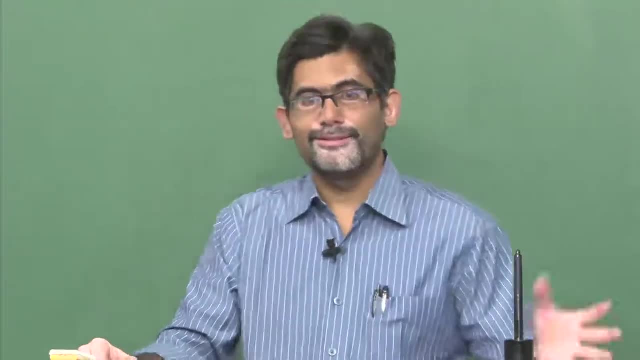 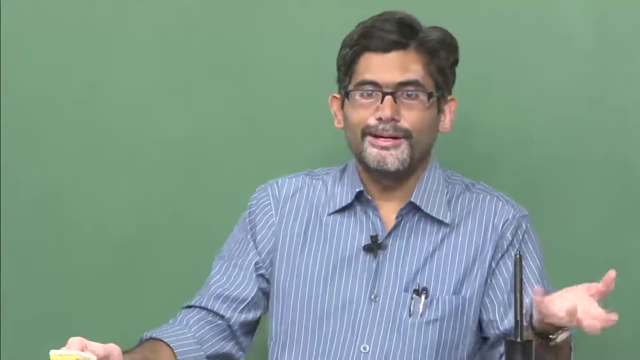 find a proof. Suppose, if I give you a contradiction, then ask you to prove, and there is no way in which you can prove that particular kind of contradiction. but if I give you a tautology like P or P, P or not P, etc. obviously you can find a proof for that. so now, these are some of the important. 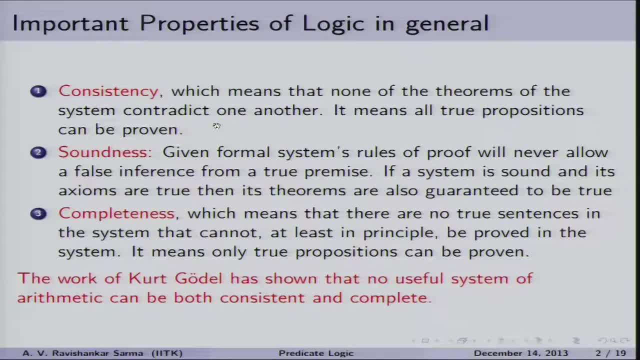 virtues every logicians would dream of. but we will be seeing very soon that in the works of good Godel he showed that no useful system of arithmetic. Godel was looking for this interesting properties in the context of arithmetic. he could find an important result, that is incompleteness theorem, with which he could say that no useful 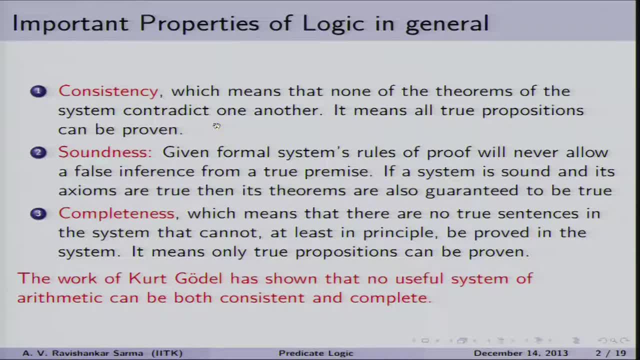 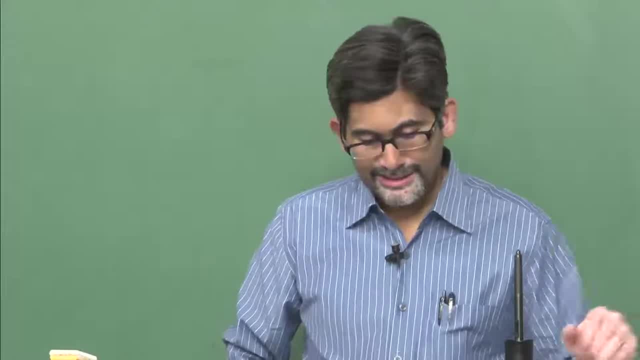 system of arithmetic can be both consistent at the same time. it can be complete. So it has to be inconsistent to be complete, or it has to be incomplete to be consistent, etc. these interesting things that you will see little bit later. so now we will be focusing. 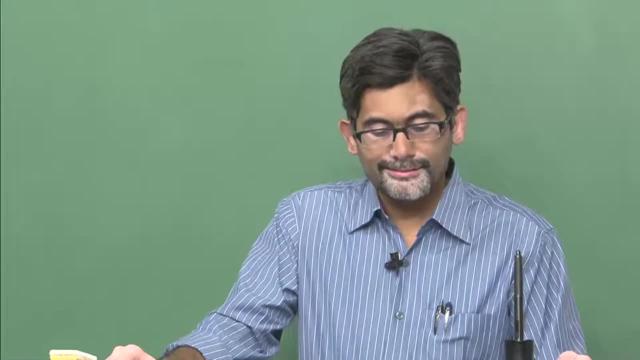 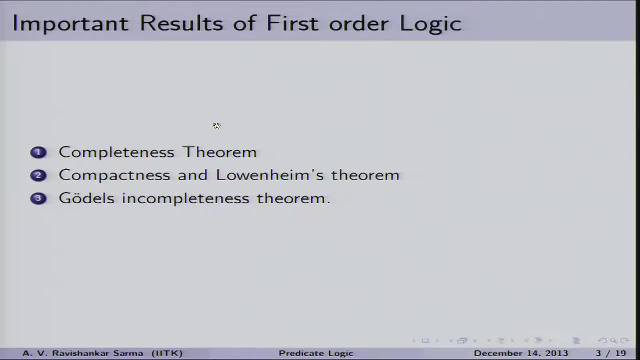 on three important Theorems: first is completeness theorem, second is compactness theorem, which has this consequence to another important logician, Loewenheim, Scholem, Loewenheim's theorem, and then we will end up with Godel's incompleteness theorem and its impact on in the area of philosophy. 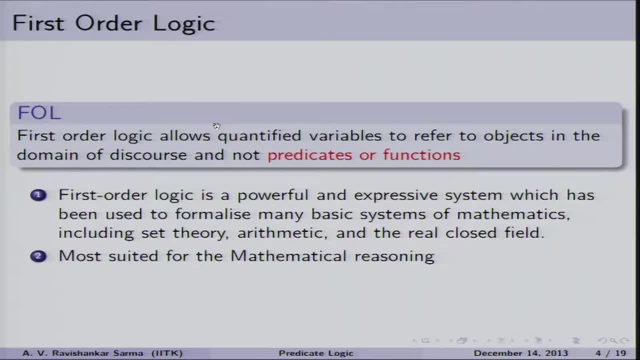 So before going further, just we need to know something about the first order logic. so when we say first order logic, it means this first order logic only allows quantified variables to exist. So quantified variables are the variables to refer to objects in the domain, in the domain. 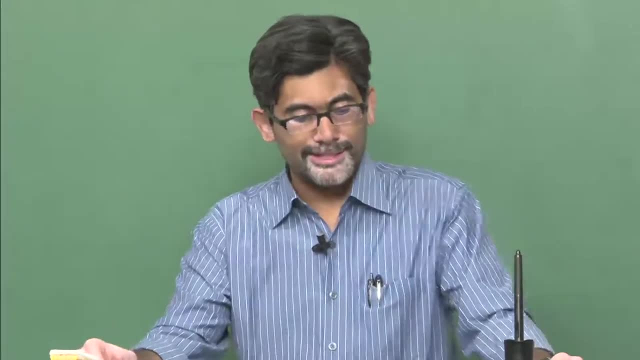 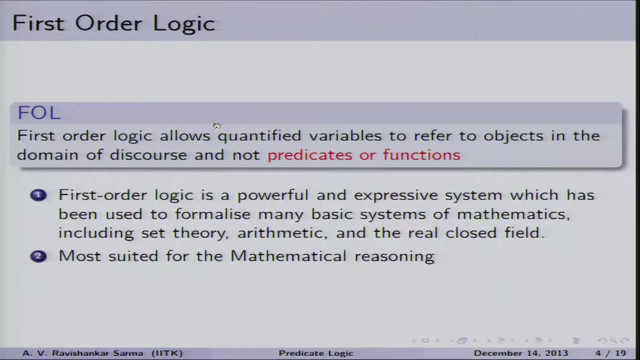 we have objects, predicates, functional symbols, except right now. so the quantified variables refer to only objects in the individual, in the domain of discourse, but not the predicates are functions. if you also take into consideration predicates in functions etc. you are talking about higher order logics, second order, third order, except first order logic is usually. 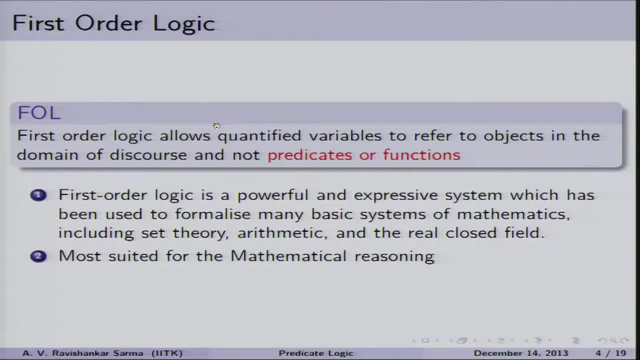 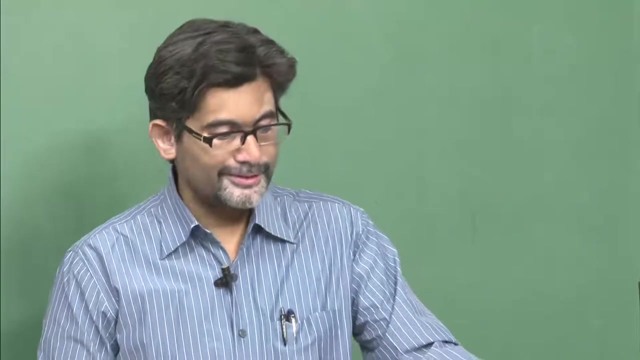 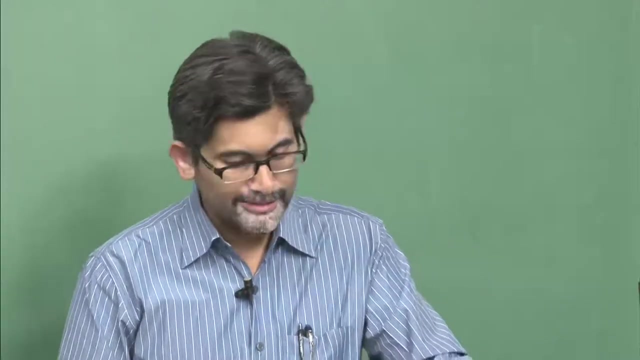 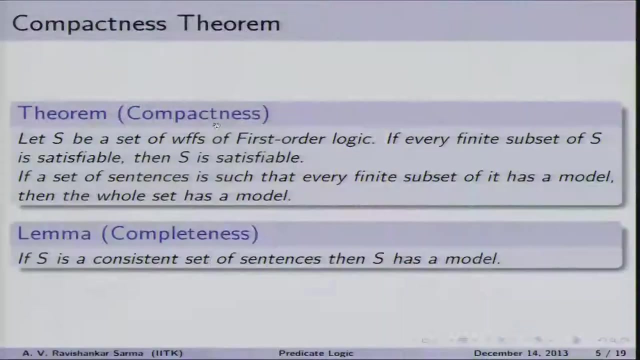 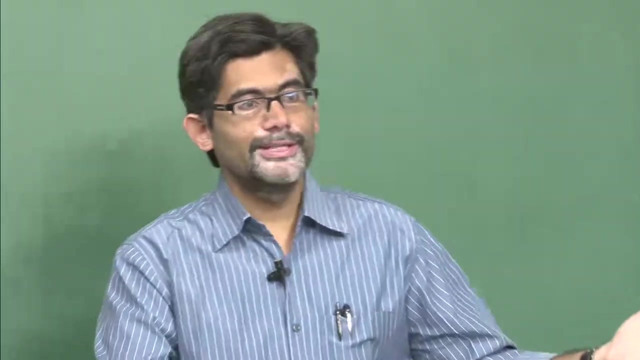 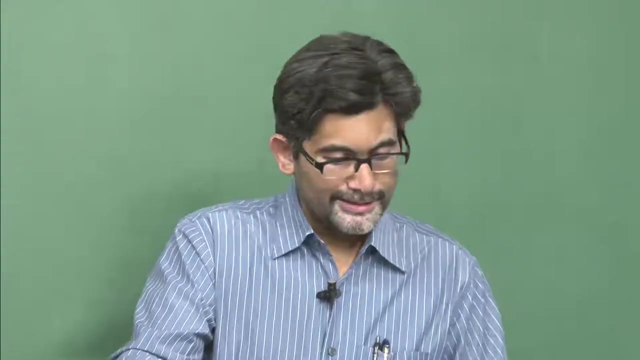 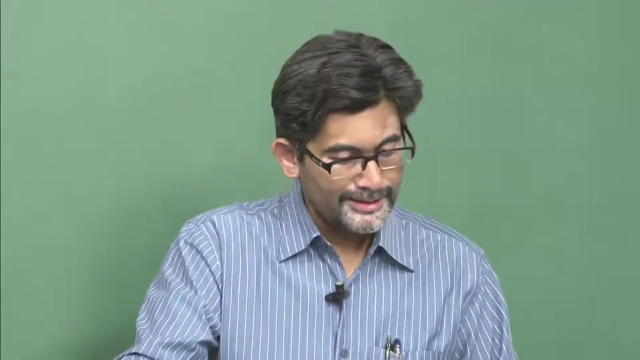 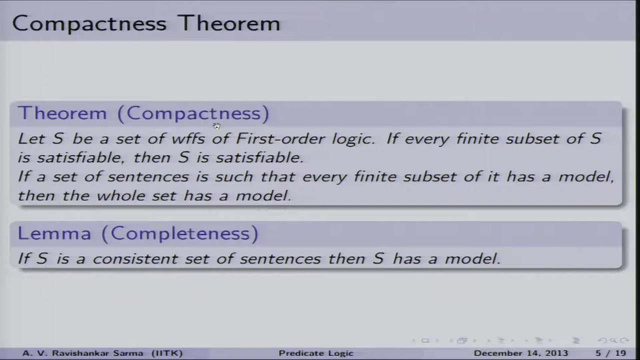 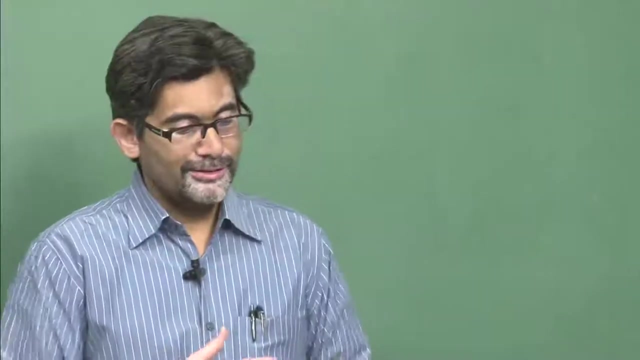 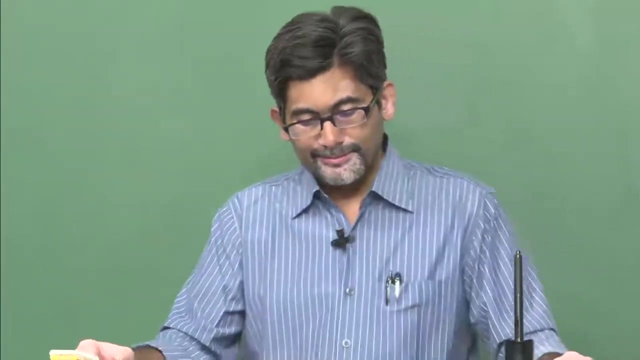 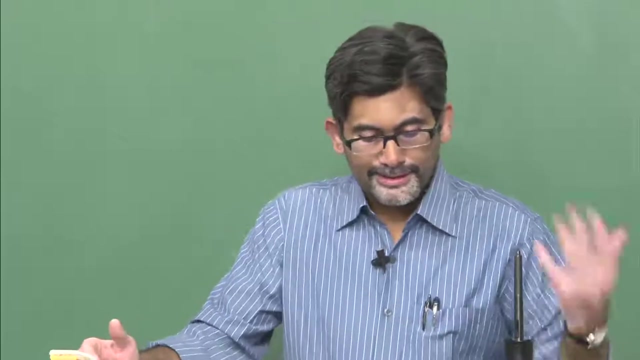 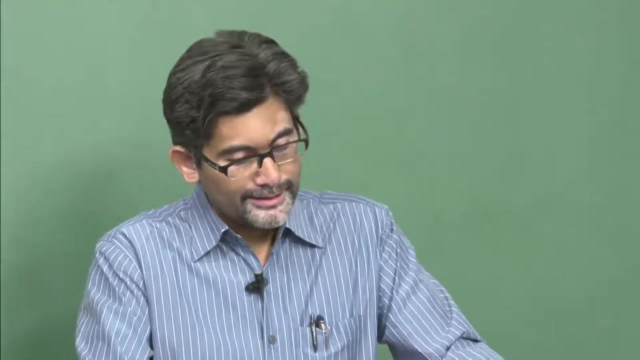 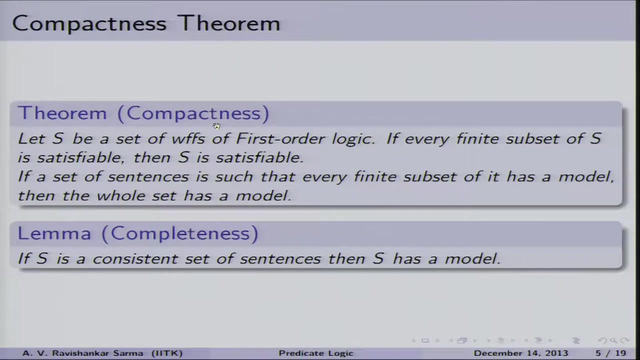 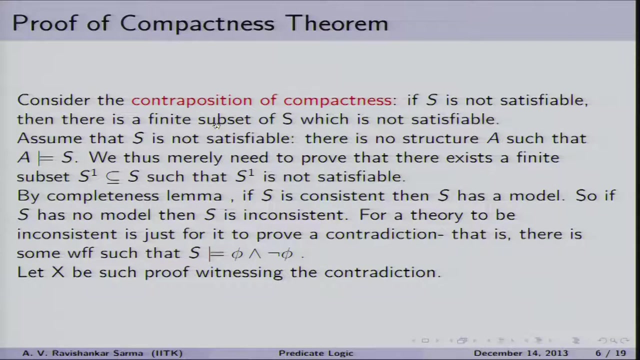 considered to be powerful and expressive system. So lemma for this one compactness theorem is this thing: if S is consistent set of sentences and obviously S has to have a model, So proof of compactness theorem goes like this. just I am giving you a general description. 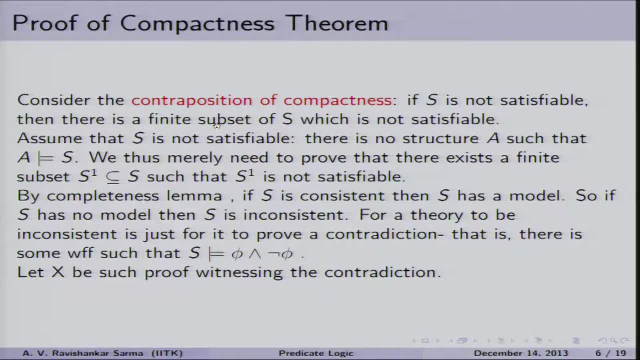 of proof. so you need to note that each and every theorem should have, should find, a proof and all. although I am not producing proofs of all the theorems that I am trying to discuss, my intention is to talk about only the general idea of these proofs, where it is later we 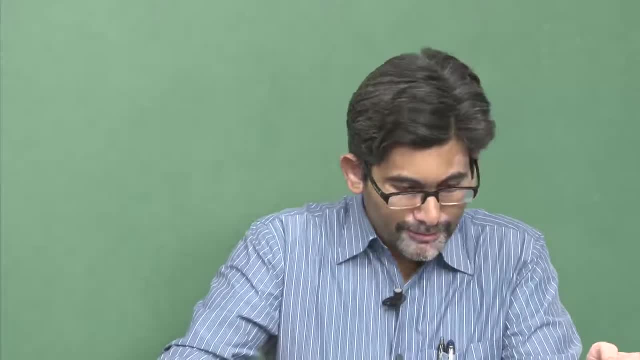 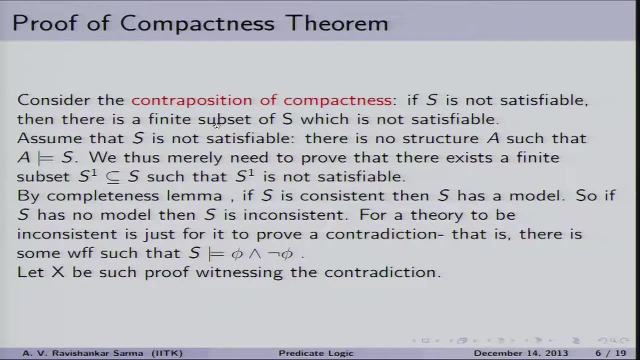 can see. So proof of compactness theorem goes like this: let us consider the counter position of compactness. that means you take the negation of the statement that you have seen the theorem of compactness. that means if S is not satisfiable, then there always exists some kind of finite. 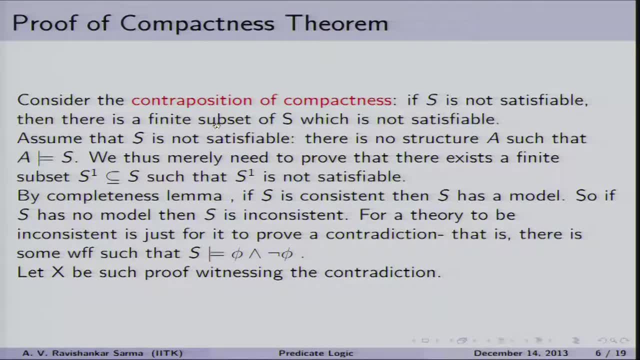 subset of S, we S1, S2 or anything, and that also should not be satisfiable. and all if all, each and every finite subset is satisfiable and S is considered to be satisfied. you suppose if one of the important use of this comparison theorem is that, if you can, 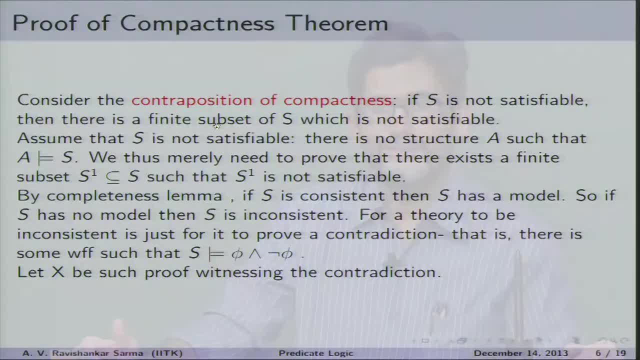 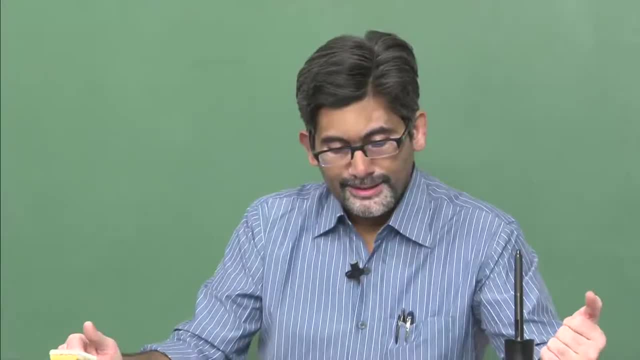 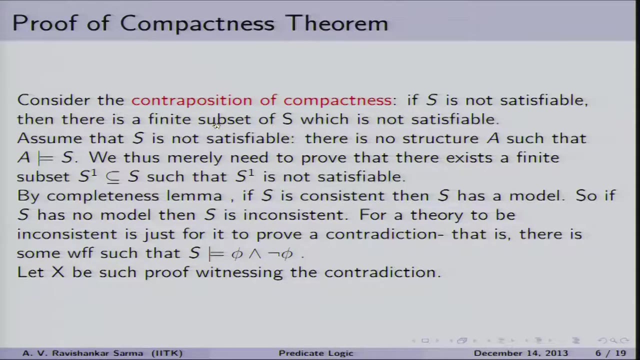 check the satisfaction with respect to subsets of a given set that will serve our purpose. So now let us assume that S is not satisfiable. that means, in the context of predicate logic, we need to have a structure A such that S is not a logical consequence of A modals S. 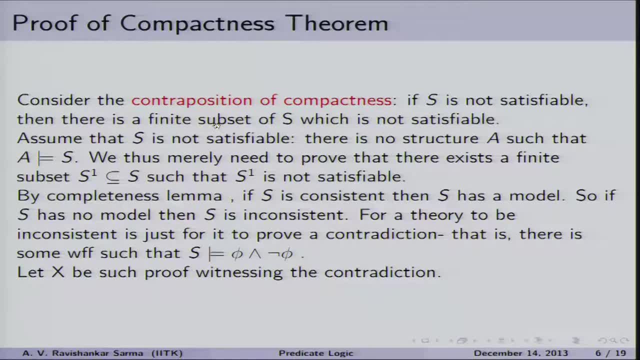 We thus merely need to prove that there exist a finite subset, S, which is a subset of S such that S is not satisfiable. So now we have a completeness lemma which says that if S is consistent, then obviously S has to find a model. so that will make use of it here, and we say that so if S has a conflux, 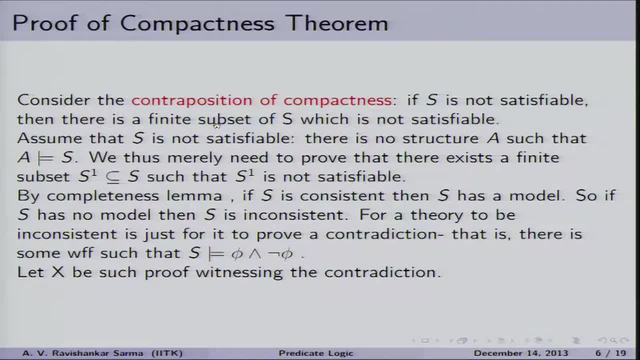 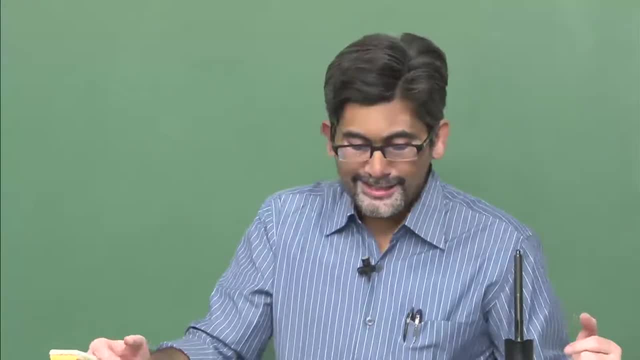 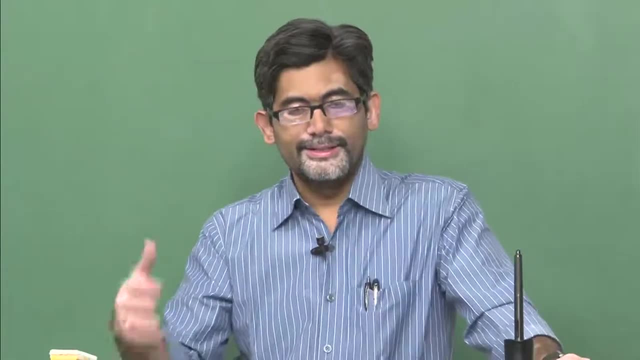 has no model, then obviously S has to be inconsistent. if you do not find any model of that one, obviously you know in all the interpretations that formula is false. that is why it is considered to be inconsistent. so for a theory to be inconsistent is just for it to prove that it leads to some. 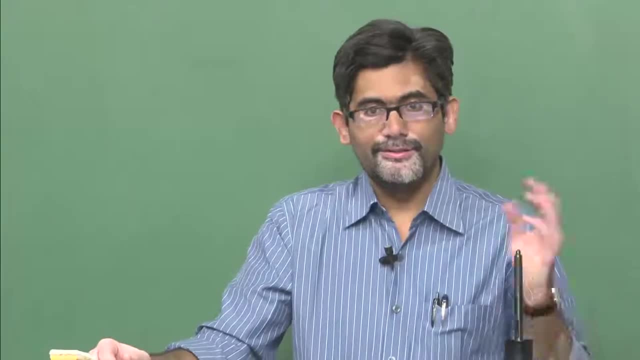 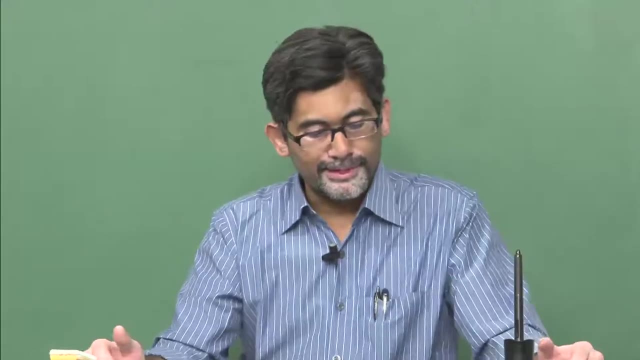 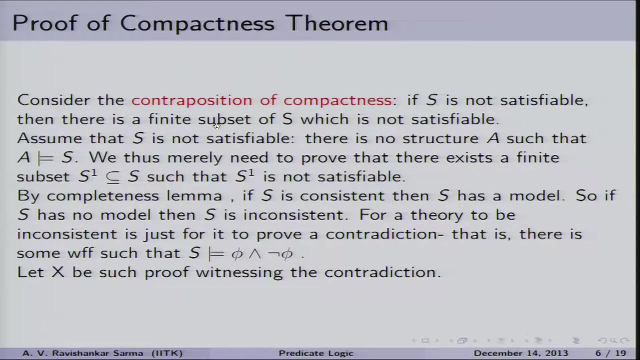 kind of contradiction that means you have come up with the case where you have a formula and its negation as an outcome of your that particular kind of set of well-formed formulas. that means let that particular kind of proof, which consist of this contradiction, be a sequence. 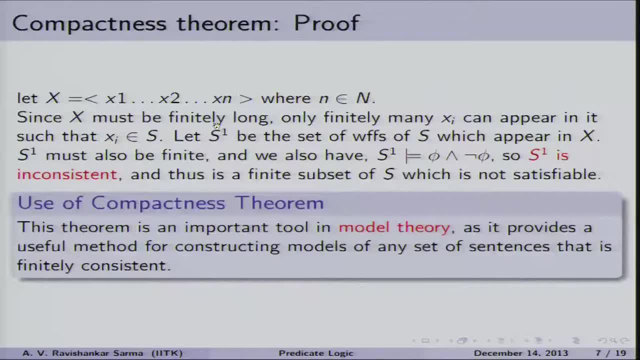 of steps, which is represented by X, so that X has this thing: first step is X1, X2, Xn and the n step is something like Phi and not Phi. there is a contradiction that you got in your proof Where n is equal to 0.. 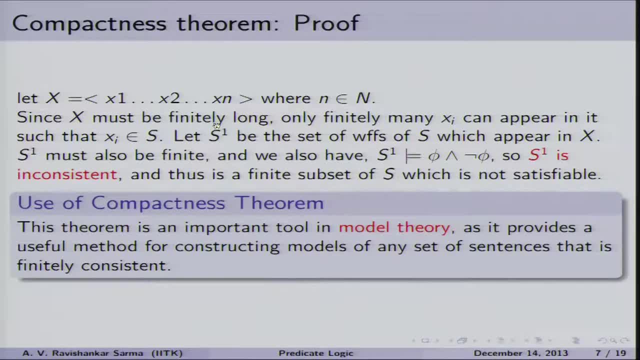 N stands for n is a natural number. that means in the finite steps. this proof ends. that means since X must be finitely long and only finitely many, excise can obviously appear in it. so that means you came across some kind of contradiction. that means you could have got it through finite. 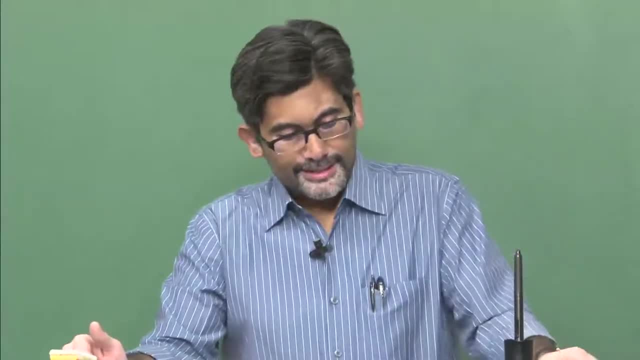 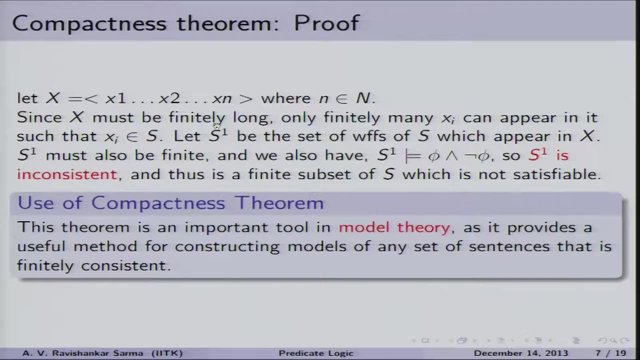 number of steps in, so such that excise, some excise that you take into consideration, which has that particular kind of contradiction that belongs to S. now, let S prime be a set of well-formed formulas, S, which appear in the proof that you are trying to talk about, where you have a contradiction. 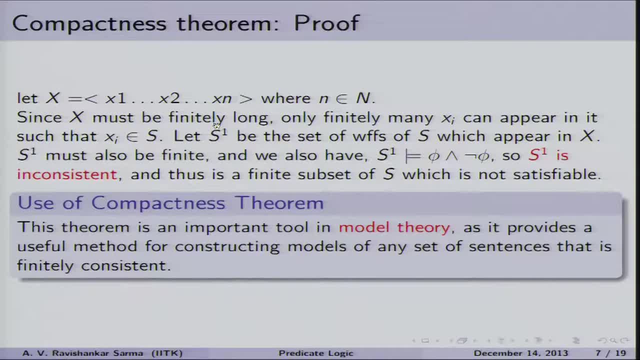 then S prime should also be finite, like the one which we have. we have seen in the case of S. that means we also have Phi and not Phi, which is which comes as an outcome of S prime. that means S prime has to be inconsistent and thus the fine and even the finite subset. 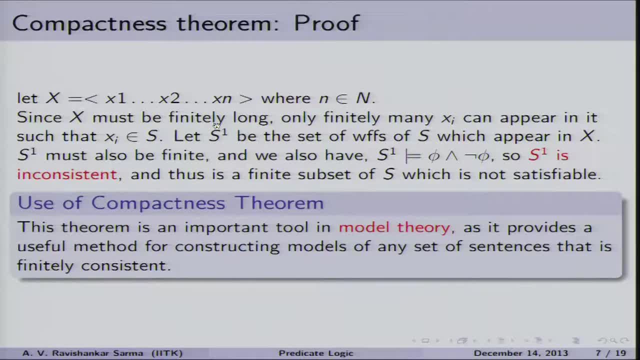 is, S is also considered to be not satisfiable. So what the idea is? S prime is a set of well-formed formulas which appear in the proof that you are trying to talk about. where you have a contradiction, then S prime should also be finite, like the one which 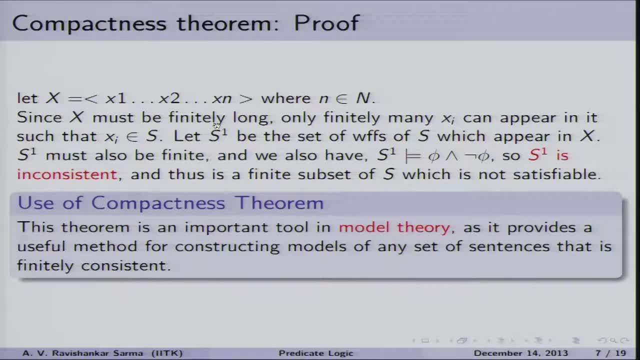 we have seen in the case of S prime. So the essential thing that you need to note is that you want to show that S is not satisfiable. you can show that you can take some finite subset of S and you can show that it is not. 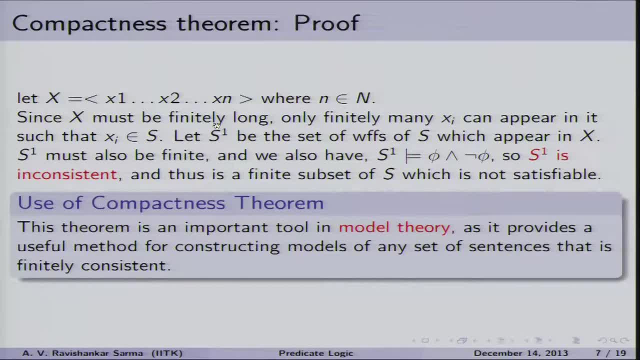 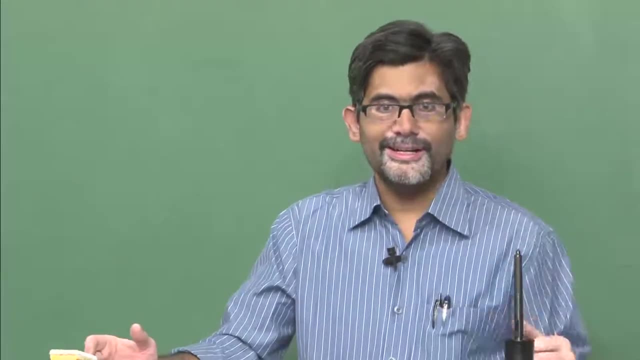 satisfied. that will serve our purpose. in that sense we call formal system to be compact. each and every finite subset of S has to be consistent or satisfiable so that the whole set is going to be satisfiable wherever one particular kind of subset of S is not satisfiable. 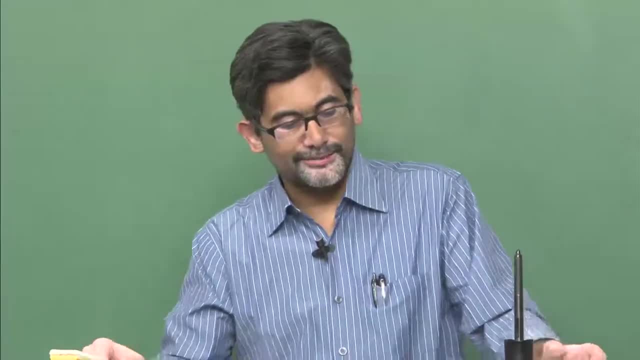 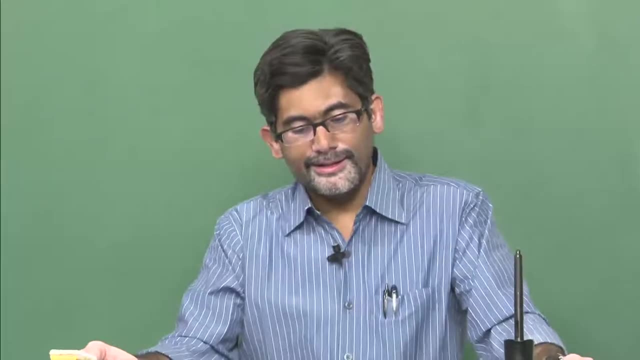 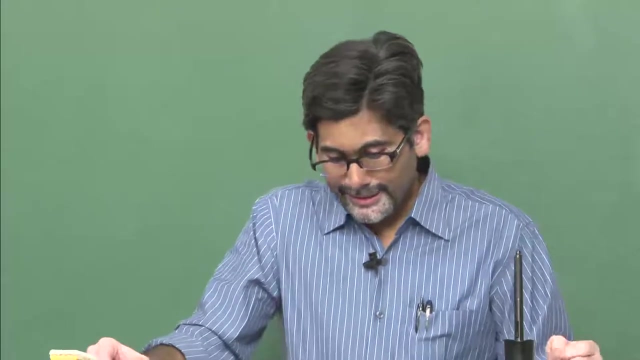 Then the whole set S is not going to be satisfied. what is the use of companion serum? this theorem is considered to be an important tool, especially in the context of model theory. model theory is important branch in the area of mathematical logic. it provides us with the useful method. 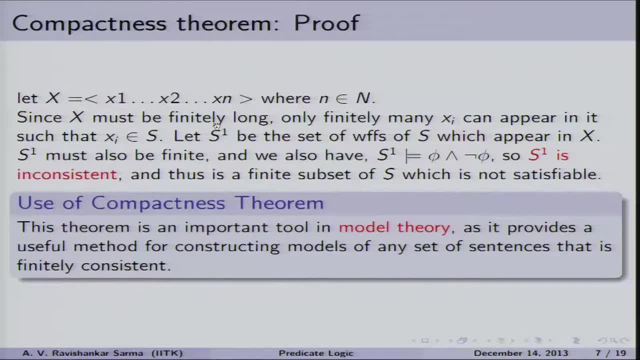 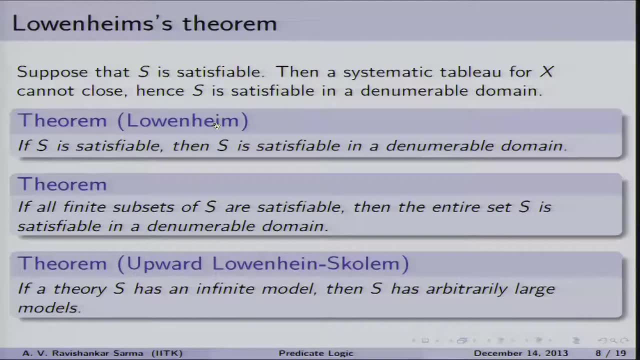 for constructing models of any set of sentences that is finitely consistent. So it is one of the important applications of this compactness theorem. Now let us talk about another important and interesting result in the first order logic, that is Lowenheim's theorem. suppose you take SS to be set of well-formed formulas. that 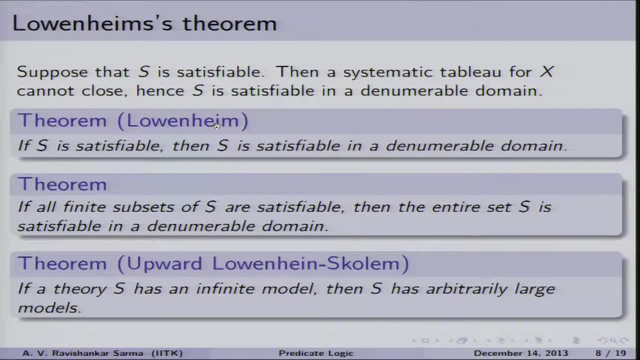 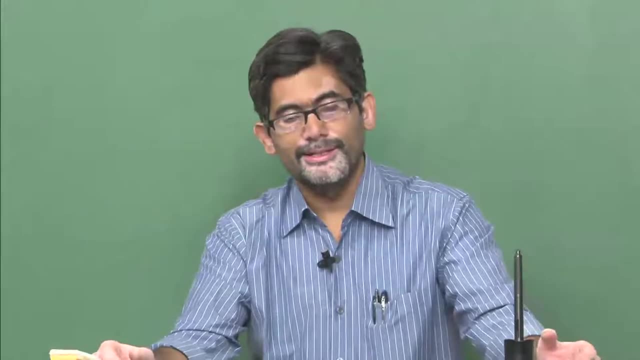 is considered to be satisfiable. that means at least one interpretation that formula S is true, then obviously, if it is satisfiable, then it has to find some kind of systematic tabular for X, that S, which obviously cannot close. that means all the open branches are leading to satisfiability. means if you have, if you have a formula in the predicate logic. 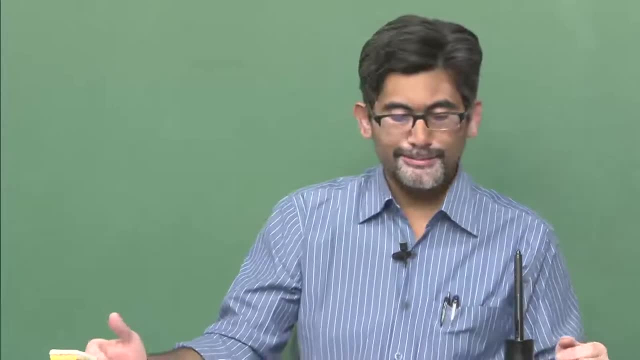 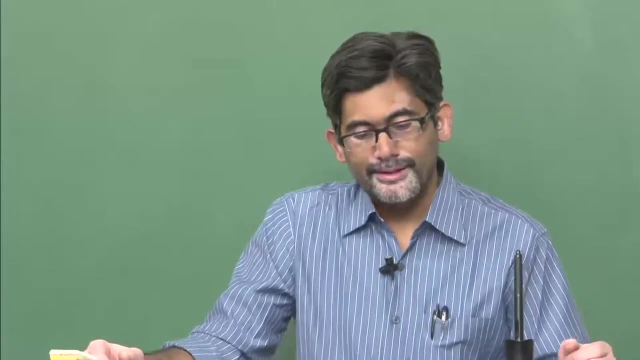 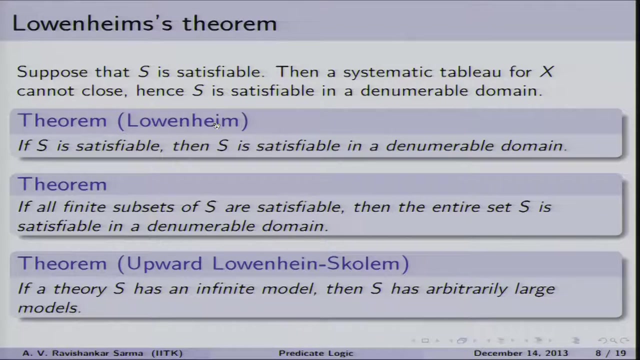 you consider a tree diagram and you have open branches. that means that open branch tells us that the given formula is satisfiable in that particular kind of interpretation. that means S has to be satisfiable in a denumerable more domain. So let this Lowenheim's theorem tells us this thing: if S is considered to be satisfiable, 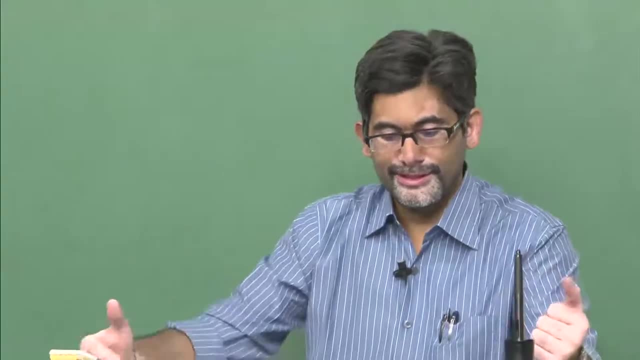 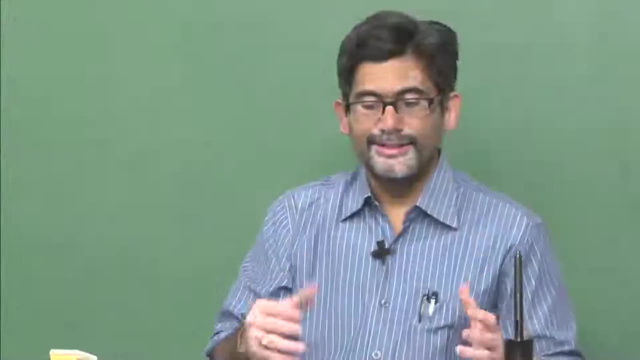 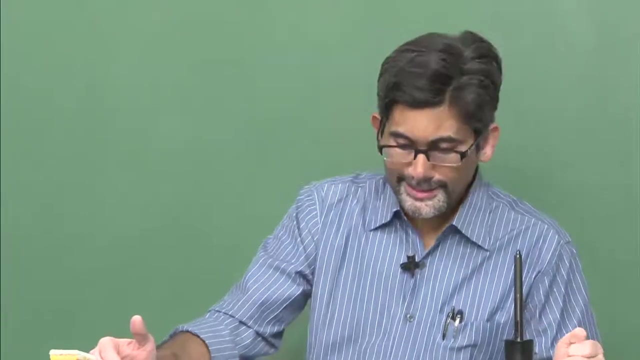 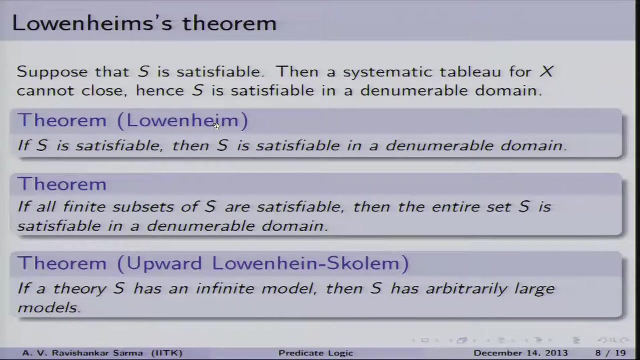 that means it finds an open branch after Using the tree rules. then S is satisfiable in a denumerable domain. that means you can number of steps would be finite in number. or it is satisfiable in a denumerable domain and the corresponding theorem is this thing: if all finite subset of S are considered to, 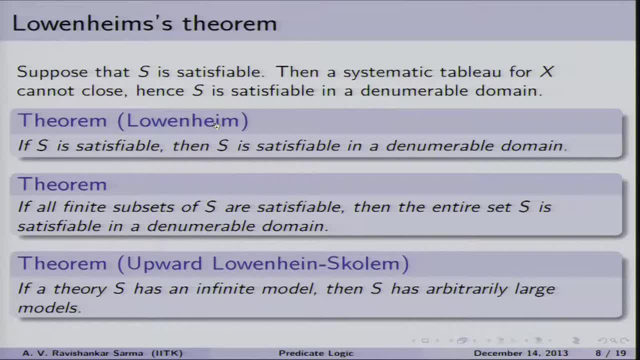 be satisfiable, then the entire set is considered to be satisfiable in a denumerable domain. So there is another interesting corresponding theory theorem. in the context of Lowenheim it is called as Lowenheim's upward Lowenheim's Coulomb's theorem. so this tells us this thing. 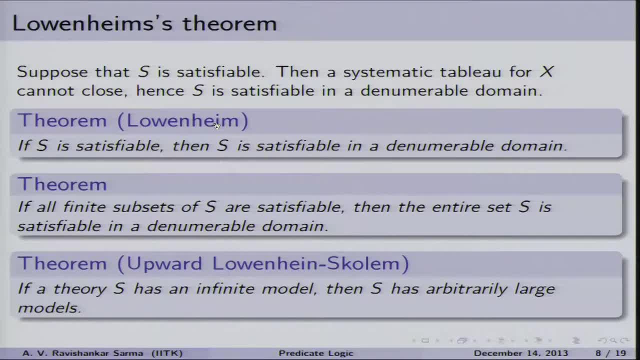 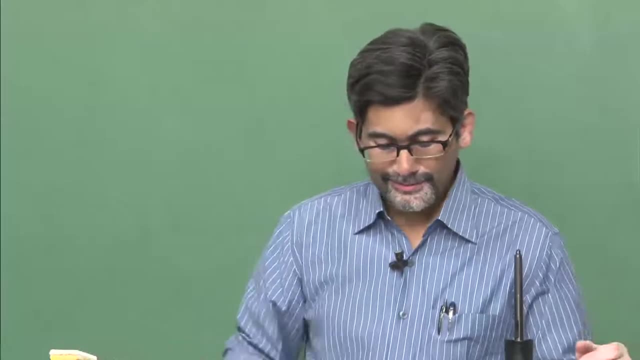 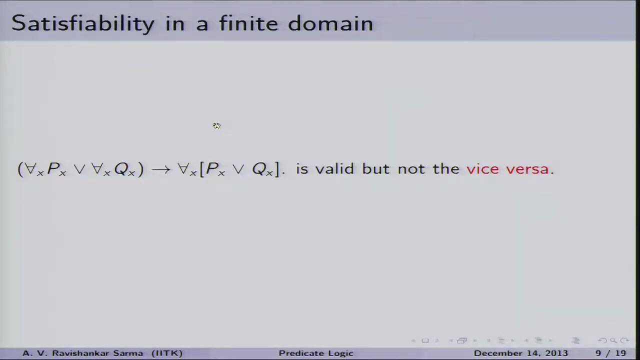 if a, if a theory S, the formal system S, has an infinite model, then S this particular S has arbitrarily large kind of models. if it is infinite model, it will have. it will take a lot of time, it will take infinite number of steps. So S has infinitely large models. for example, if you want to see the one of the applications: 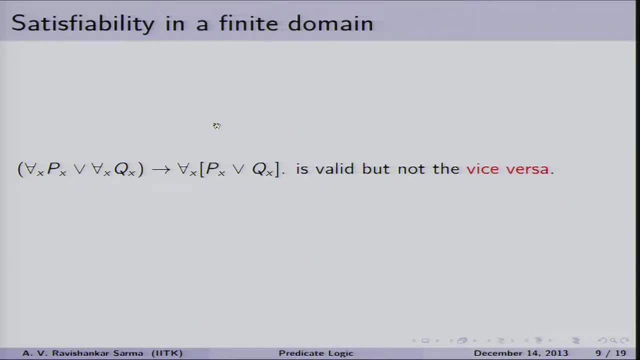 of this particular kind of for theorem. it is like this: this formula for all X, P, X, for all X, Q X implies for all X, P, X, R, Q, X is going to be tautology and hence it is valid formula. but if you take the vice versa of that one, that is, for all X, P, X, R, Q, X implies individually. 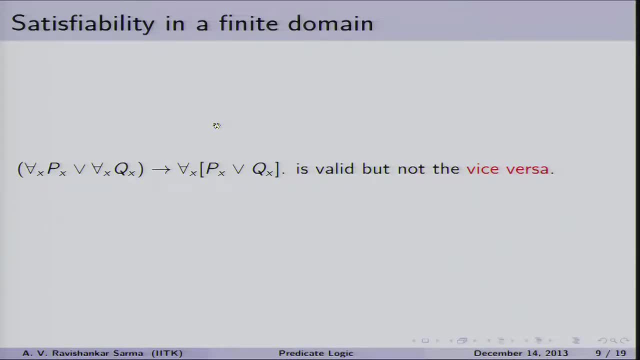 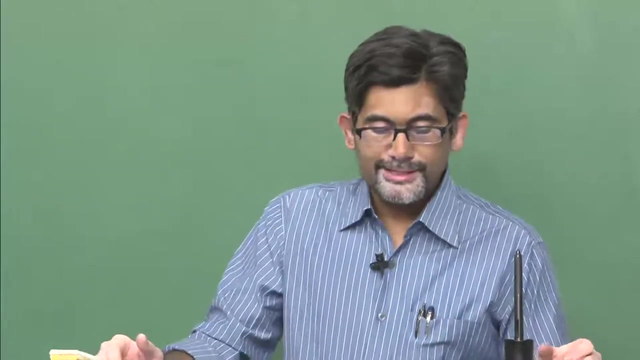 for all X, P, X, R for all X, That is considered to be an invalid kind of formula. and if you want to establish that it is unsatisfiable, and you, if you construct a tree diagram, infinite number of steps, it will end and then you will have some kind of open branches. that means if you deny the 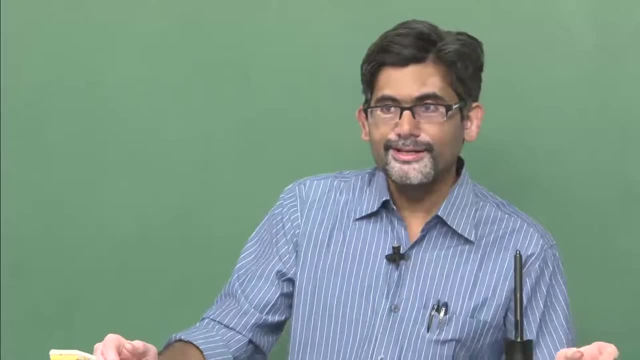 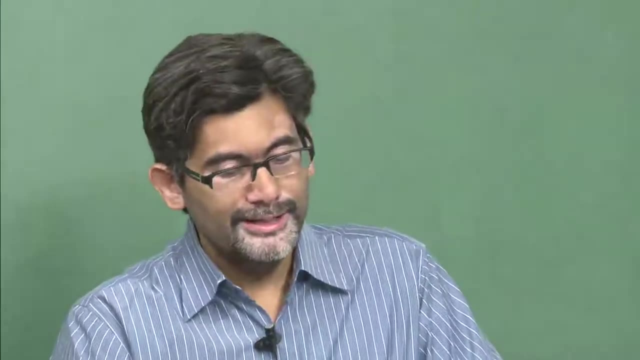 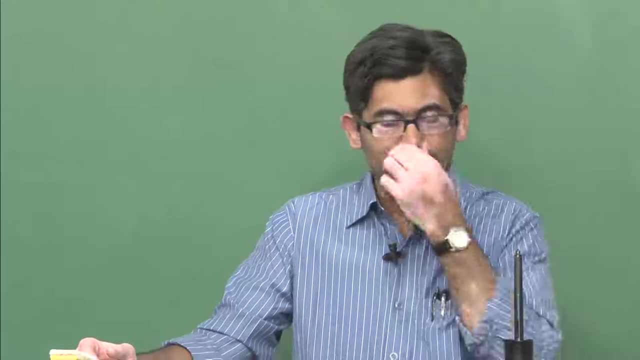 formula, you will have the open branches. this example we have taken into consideration in the last few lectures. So we can easily construct from the open branch a counter example and if you see that counter-example you will have you. you only require some kind of finite domain and all which involves one. 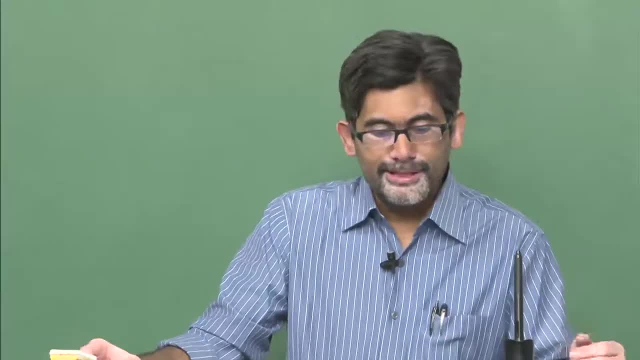 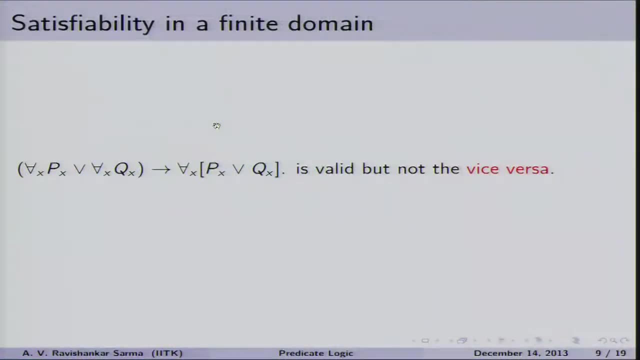 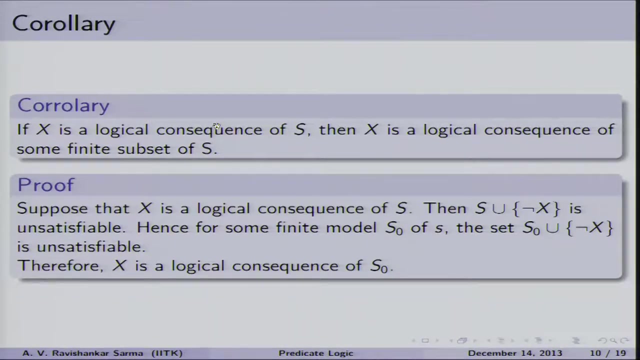 or two elements, one or two parameters on A or B to establish this particular kind of thing. So you will just require a finite domain to prove whether it is satisfiable or unsatisfiable. one important corollary of this particular kind of theorem is this thing: suppose, if X 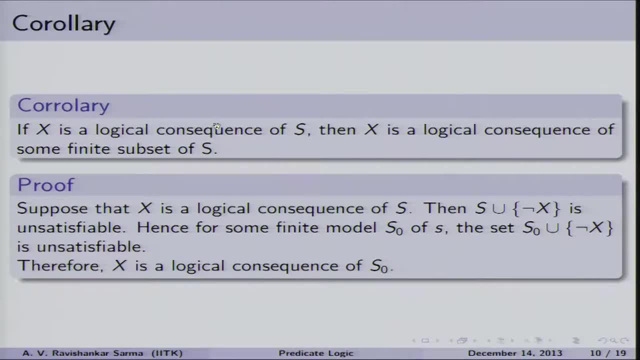 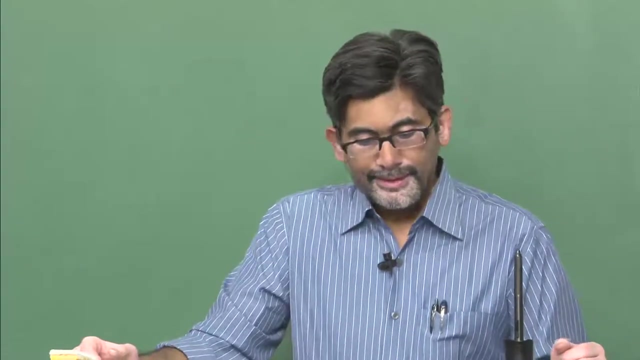 is a logical consequence of set of well-formed formulas, S, Then X is also considered to be logical consequence of some finite subset of S. So you have some large set of set of formulas and then S one consists of some kind of set of formulas which are subset of this particular kind of S. then if X is a logical consequence, 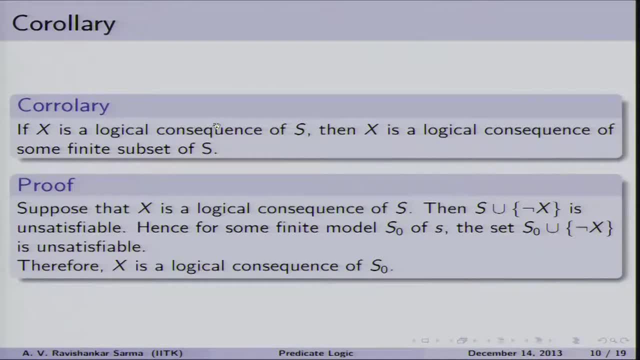 of S, then X is also logical consequence of some finite subset of S. so how do we prove this particular kind of thing? A proof goes like this: suppose that X is a logical consequence of S. that is what is given to us. that means if you add not X to S, that leads to unsatisfiable. that means if something 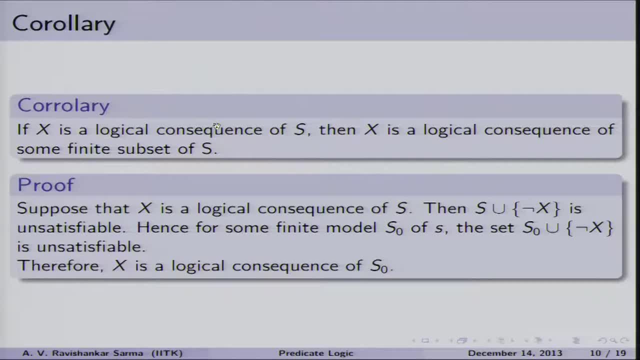 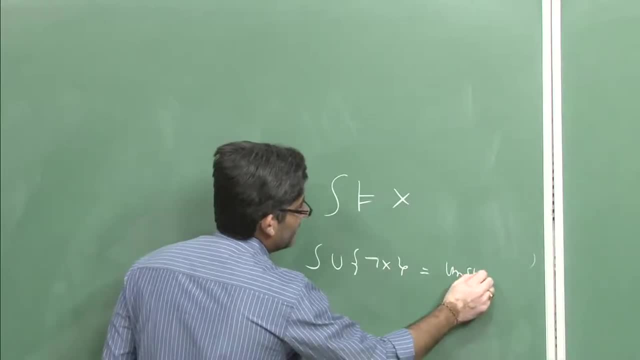 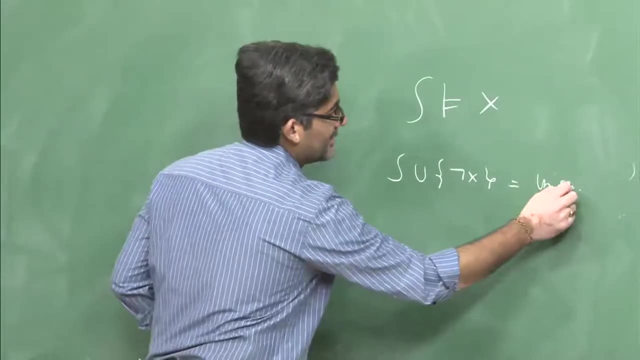 is this particular kind of thing. S is X, then if you add not X to it, then this becomes unsatisfiable. you started with the premises and you deny the conclusion, So obviously it leads to contradiction. that means it is unsatisfiable. so S union, not of. 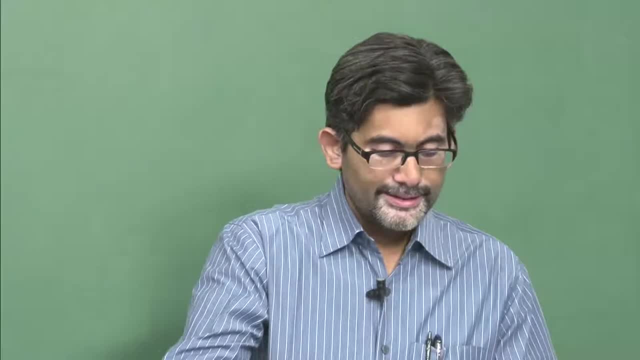 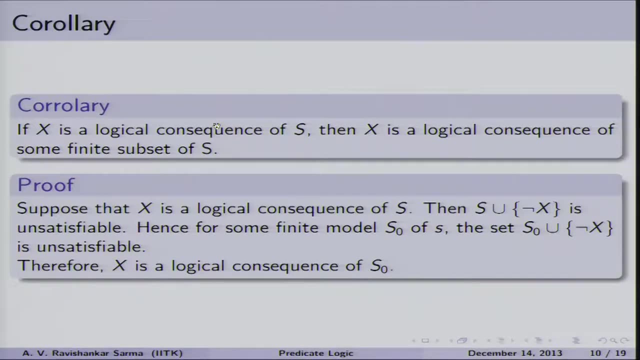 X obviously has to be unsatisfiable. hence, if it is unsatisfiable, then if you constructed a tree diagram using tabular proofs, obviously it ends in finite steps and all. hence it will have a finite model: S zero of S, the capital S, that is even S zero. union, not X, is also. 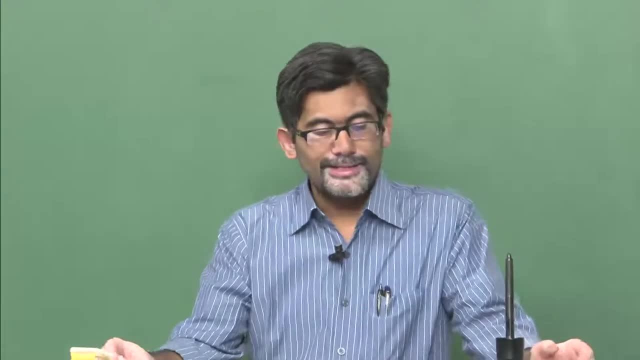 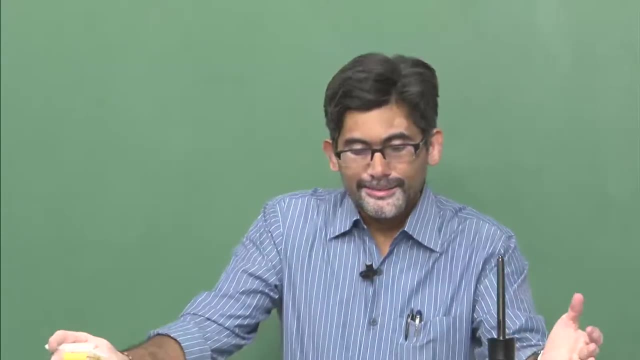 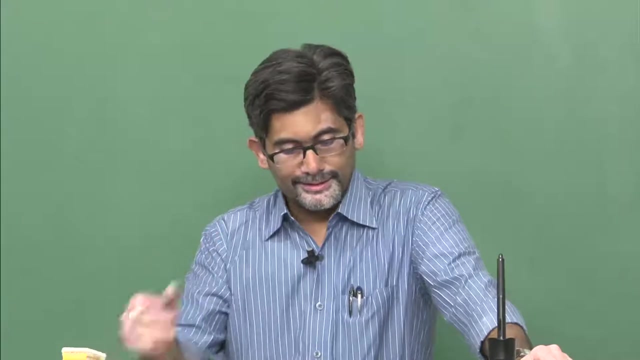 considered to be unsatisfiable. So Therefore, obviously X is also a logical consequence of S zero. so if you want to show that S is considered to be unsatisfiable, you can take the subset of S and then you can show that even from the subset of S also, that X is has to be a logical consequence. 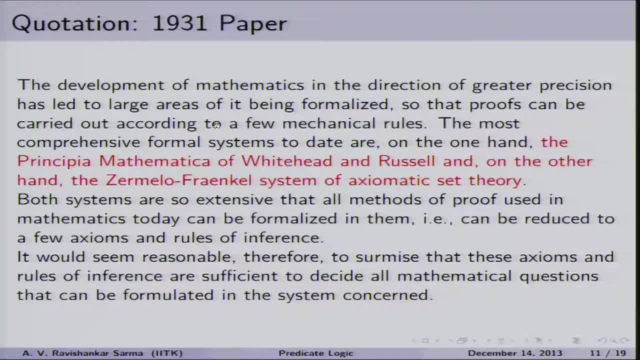 So this is what is compact. next and Loewenheim's theorem. now let us come back to the celebrated result in the first order logic: That is the golden theorem. Now let us come back to the celebrated result in the first order logic: that is the golden. 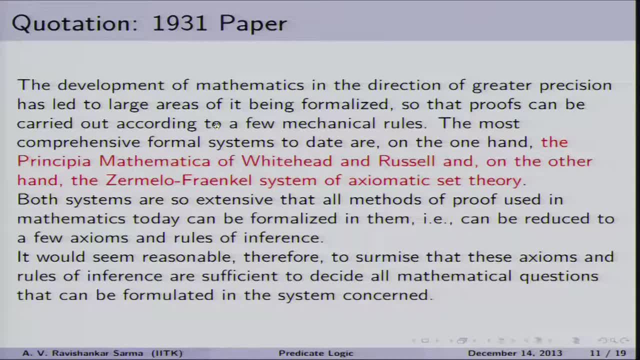 income in a serum. before talking about golden income in a serum, let us talk about this particular kind of startling kind of passage, which you will find it in one of the important and path breaking papers by Gordon. it is on some kind of formally undecidable propositions. 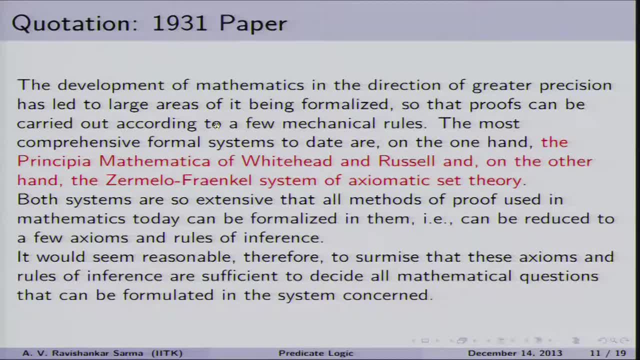 So here is an important question which is worth discussing. so Gordon says this particular kind of So he is of the view that he says the development of mathematics in the direction of greater precision has led to large areas of it being formalized so that proofs can be carried out. 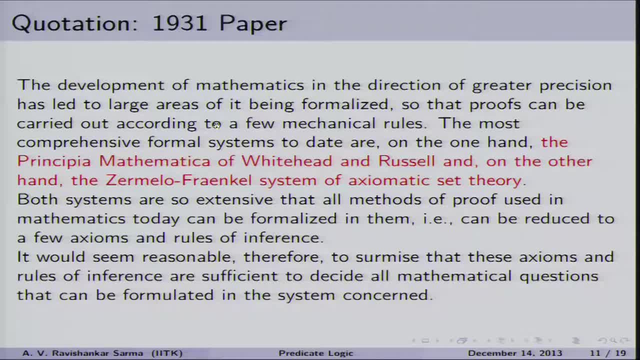 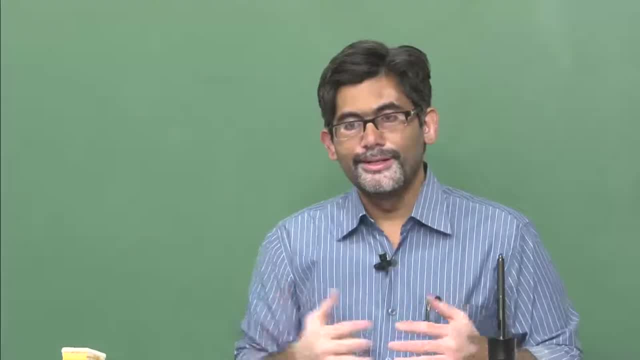 according to just few mechanical rules. that means you started with few axioms. that is what we have seen in the case of for a cell weighted axiomatic system or Hilbert Ackerman axiomatic system, etc. you started with some four or five kind of rules and then you have 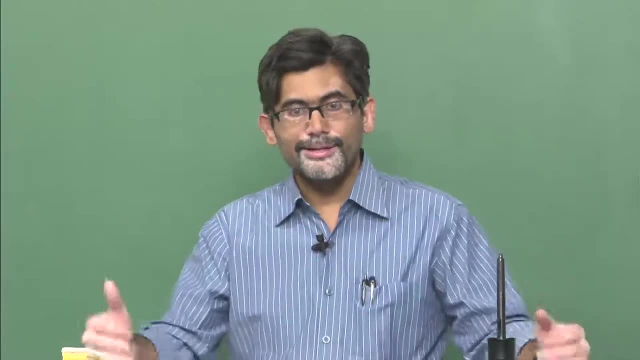 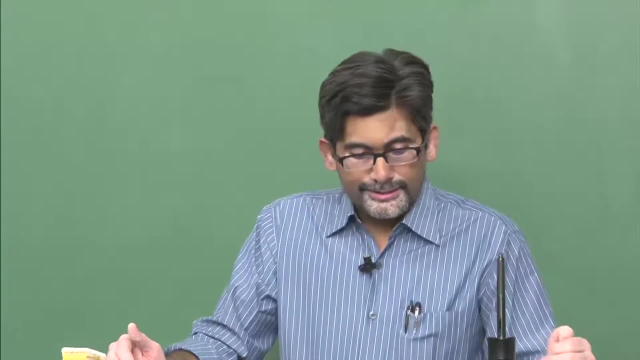 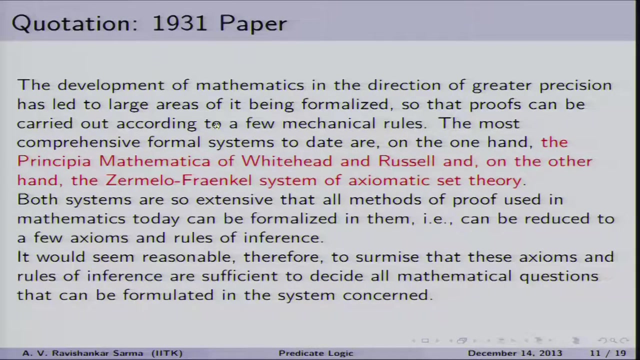 some substitution rules And some definitions, that is, schemas, and then you generated number of theorems in all, numerous theorems and all so, which just simply requires a few mechanical rules and all, and then axioms, of course, to start with the most comprehensive formal systems to date, according 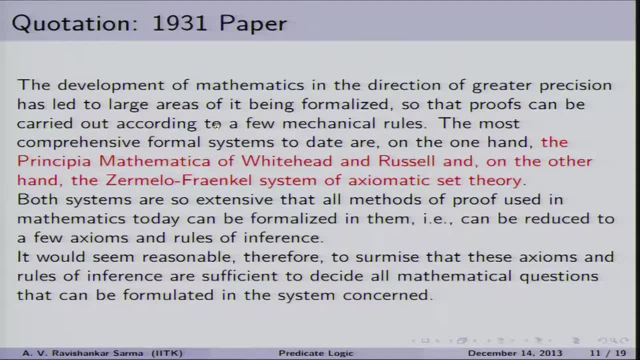 to Godel. on the one hand are these things- one is principia mathematica of Whitehead and Russell- And on the other hand We have- This is Frankl's system of axiomatic, which we did not discuss in this course, but in the